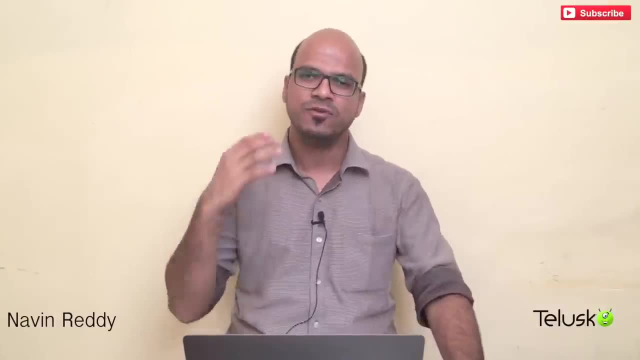 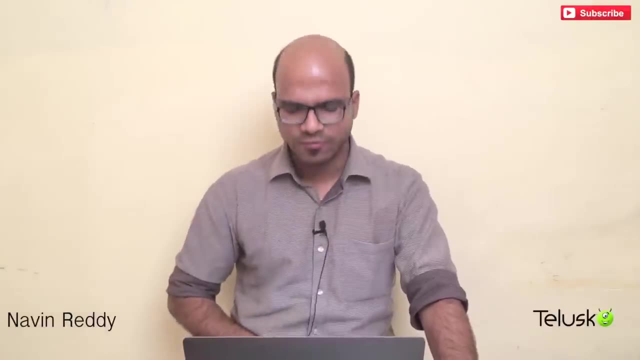 maybe it takes lots of time for creation. Let's say, if you want to create an object and that object is created with the help of database, because if you want to load some initial values, so if the object is getting created with some initial values and those values are coming from. 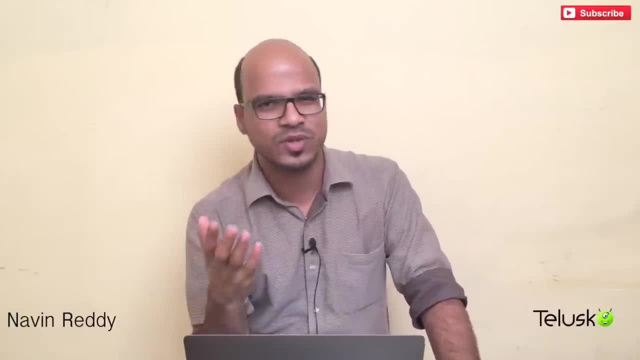 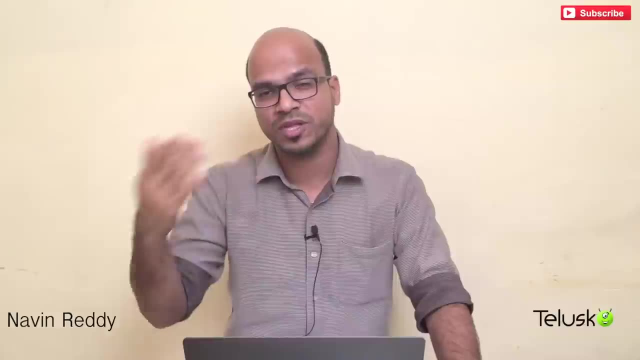 database. it will take some time. right, and of course when you create an object will take some time. But let's say, if you want to go for the second object, then why to create a new object which is communicating from the database? What if you have an object here which is? 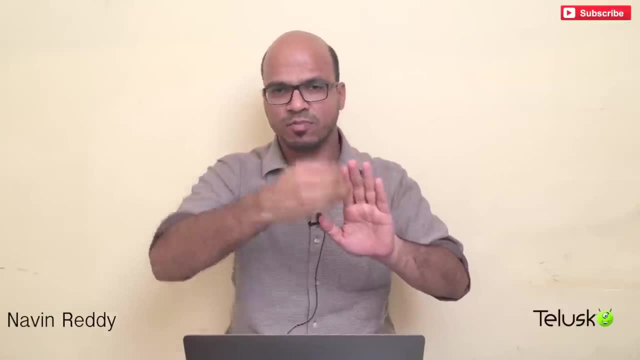 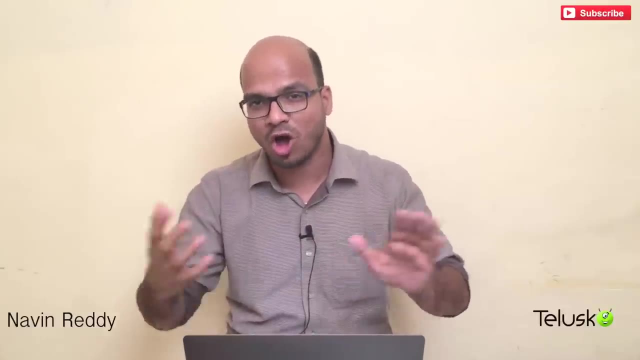 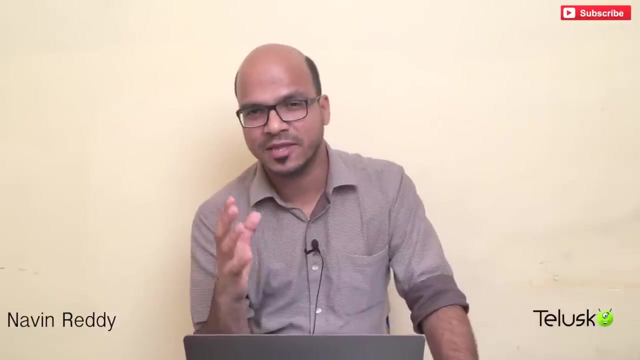 created from the database. the second object can be created from this object, right? can you just fetch the first object data into a second object? something like copying the object or something like cloning the object, right? so if you can clone the object, that is called as prototype design pattern, where 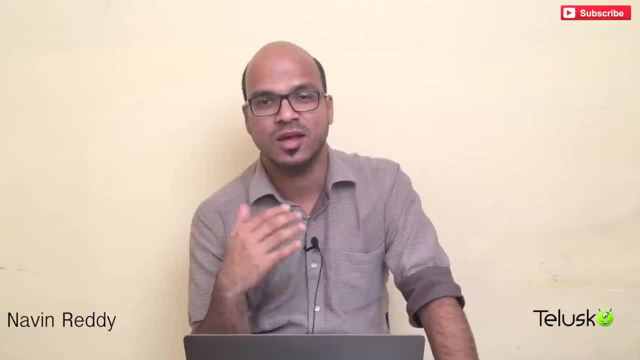 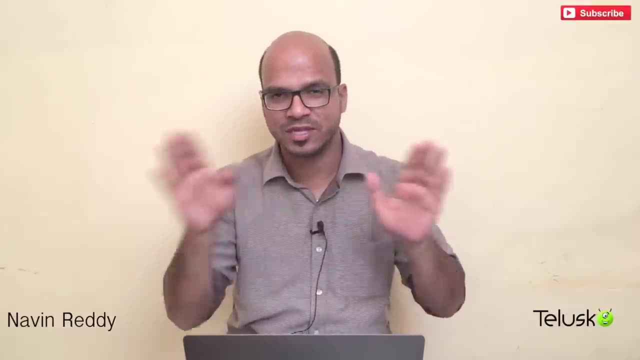 you can. instead of creating a new object from the database, you can actually use a clone concept, a cloning concept. right, because if you clone, you don't have to interact with database again. right, you can simply create an object. you can get a copy of that. it's that simple, right? so let's try to do that. let's see. 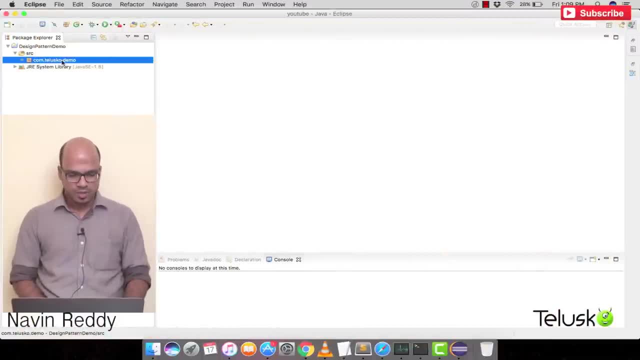 how to implement that with an example. so what I will do is I will just create a new project. so I will say: new project, and what new project? I already have a project here. we'll create a new file here and we'll say: this is okay, let's go. 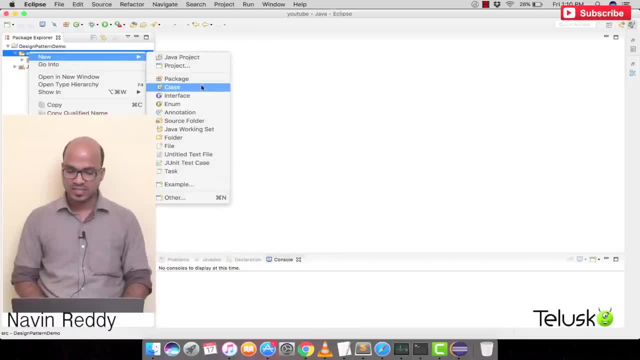 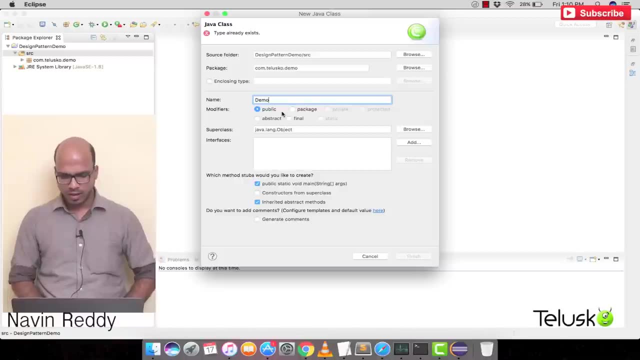 for a new package altogether. let's write like: new class: okay, and in this class we'll mention the class name as demo, because I just want a main method here. okay and okay. so let's remove this demo. we'll use a package name as prototype because we are using the prototype design pattern. let's click on finish so. 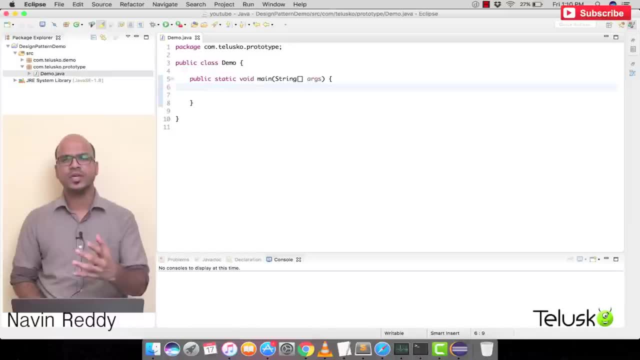 we have this main class, right? let me just delete this part. so what I want here is: let's take an example of book shop. so let's say: if you want to create, if you want to, if you want to open a book shop, so every book shop has books, of course, right? so book is a component in a book shop. so if you 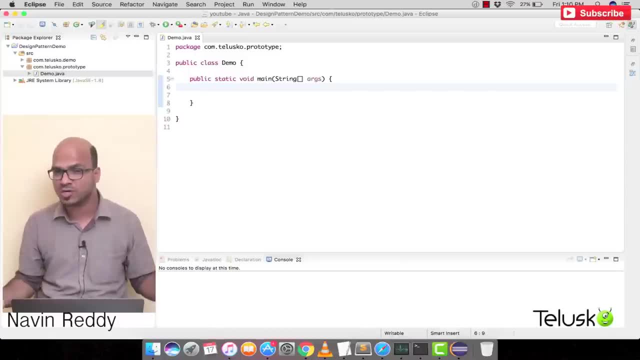 want to open a book shop, you need lots of books. right now, those books will be coming from the data warehouse. it will take some time, not data warehouse, the book warehouse, right. so it will take some time right now. if you want to open a new book shop, okay, what you can do is you can simply. 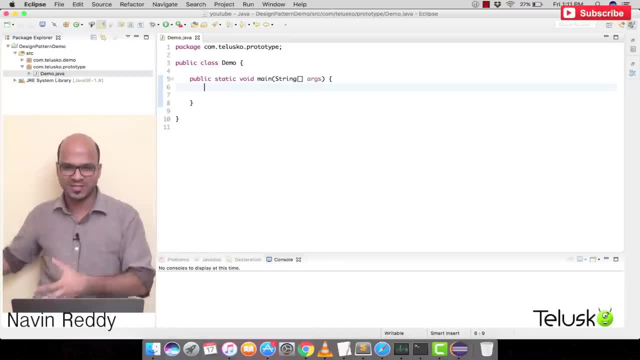 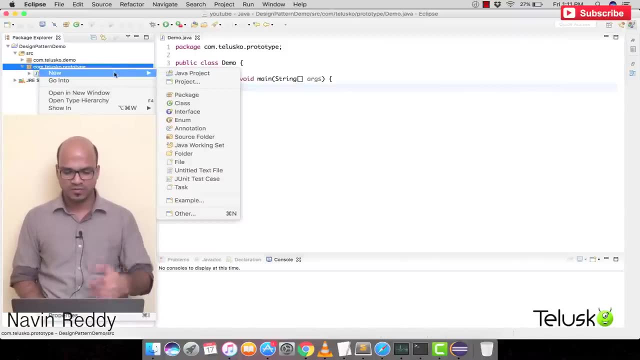 create a clone of this book shop. so you know, just copy paste. it is not possible in real world, but it is possible in virtual world. let's try to do that. so what we'll do is: let's create a book first of all. so we need a book class here. so I will. 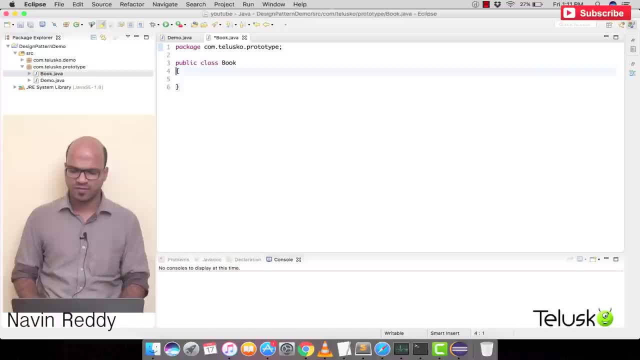 say a class book. now this book class will have, let's say, two parameters, just for the use. we'll say private int, B ID, which is book ID, and then private string, B name. so we got this two variables here. and then to access those three two variables, we need getters and setters. so I will right click source getters. 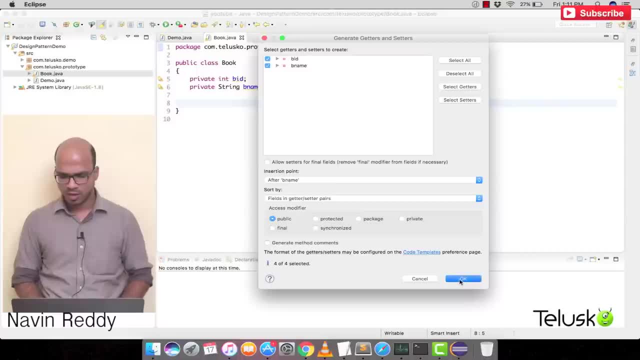 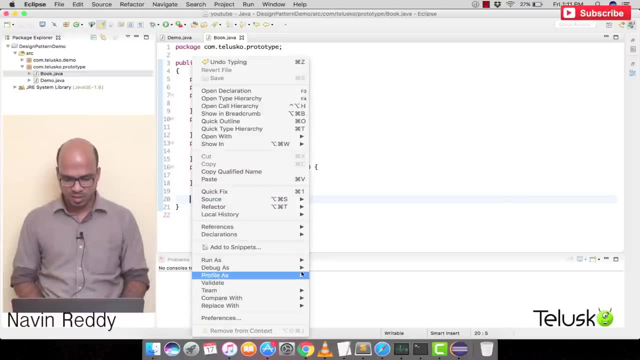 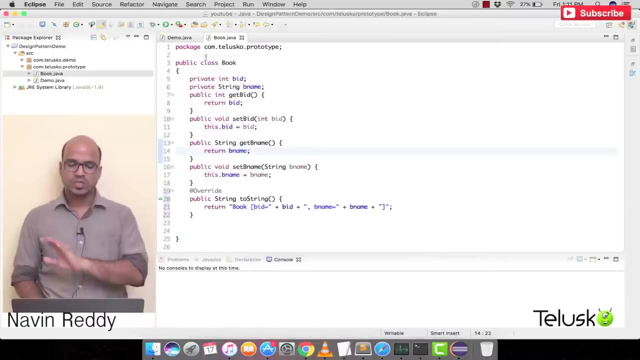 and setters will select both this variables here. click on ok, you got your book class right and let's say: let's also use a toString method if you want to print this, print this object, so we'll say source toString, which is which will take this two, and that's done. so we have created the book class now. 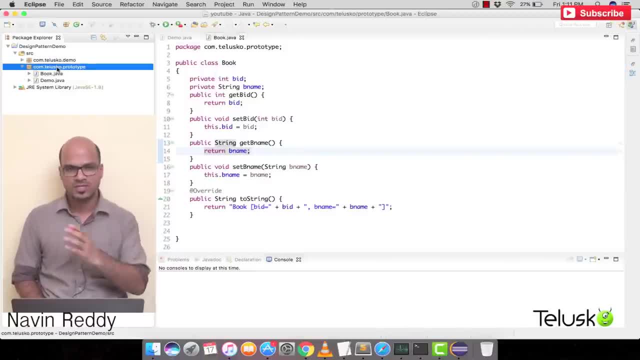 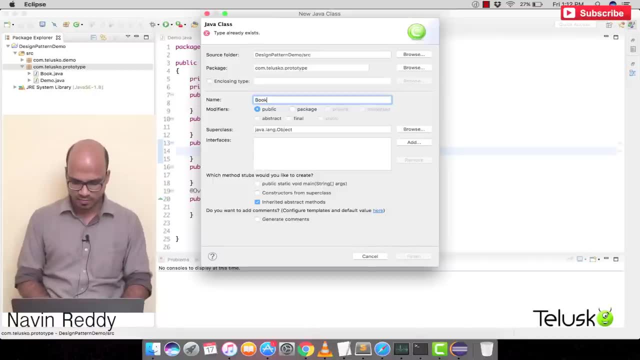 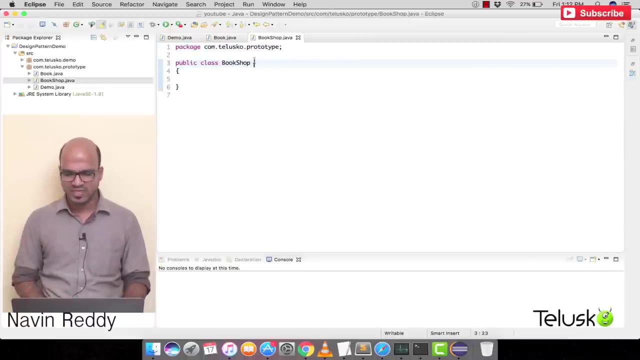 what I want is the book shop class, because a book shop, you want to open a book shop, right. so right click and say new class and we'll name this class as book shop. we'll click on finish now this book shop. what it will have is: every book shop has a name, right, so let's have a name variable here. 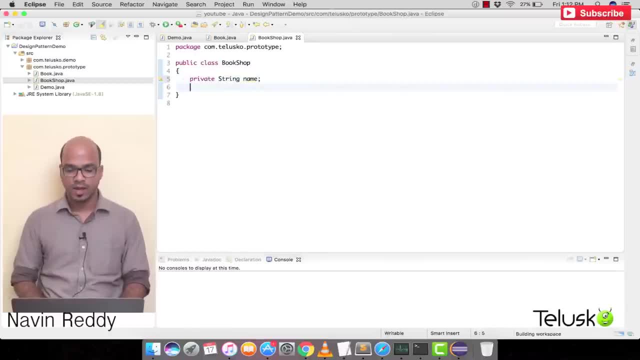 will say public, private, string name, okay, and then every book shop will have four. in fact, this should be a let's say name, or we can also have shop name. that will be more better, right? so we'll have a shop name, and then let's have one more, which is the list of books. so book. 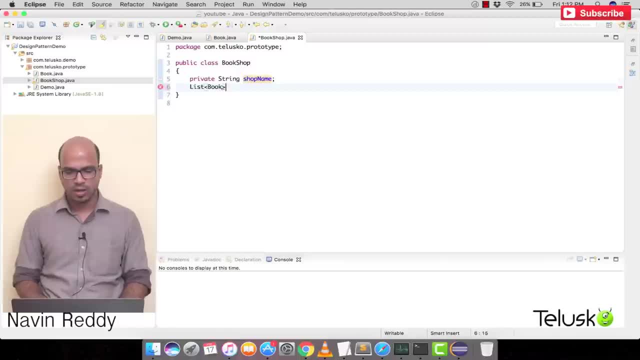 shop will have a list of books, so it will be of type book and it will be books equal to new analyst. so that is analyst and that's it. so we got books here and to access these two variables what we need is getters and setters. so we'll right click here and say source getters and. 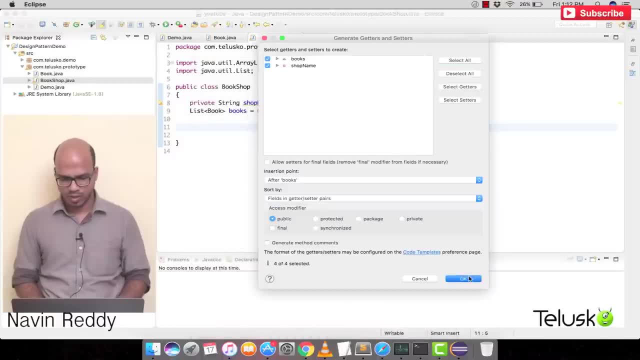 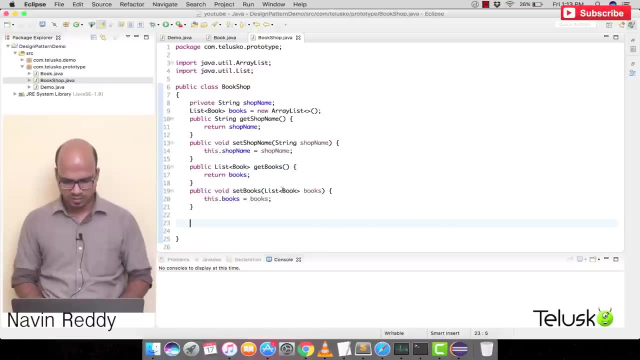 setters for this two. let's select all and click on okay, and then we will. let's also have a two string method, just if you want to print this object anywhere. so we'll say not getter, setter, but two strings. so right click source getters and setters, which is here, and oh, what i'm doing. 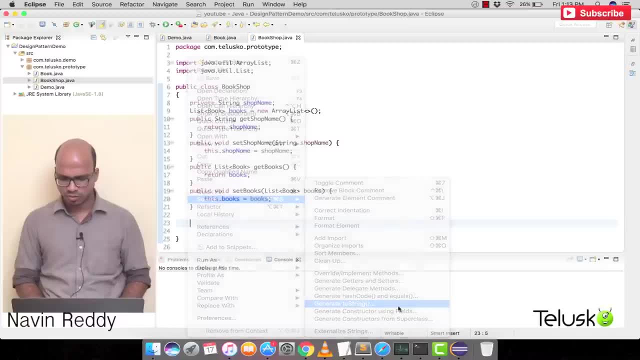 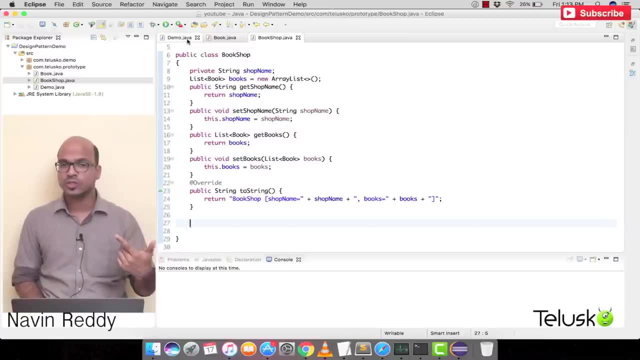 getter setter. every time it should be two string, right, so we'll say two string and click on okay, okay, so we got two string, we got books. so what i want here is i want to, okay, so let's create, let's create object of books here, and that's simple, right, not books, but bookshop, so we'll say bookshop. 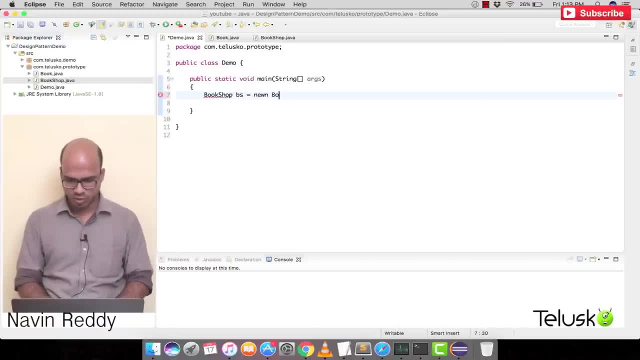 and we'll say: bs equal to new bookshop. okay, so we got bookshop there and now let's print this object. let's see if it is working or not. so i will simply print this object, okay, nothing else. okay, let's run this. you can see, we got the output, but the name of the bookshop is, i mean, the shop name. 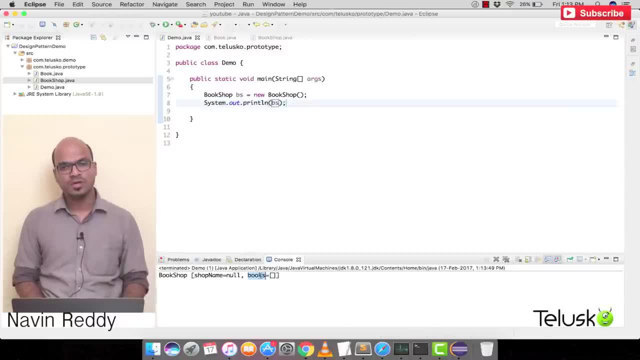 is null because we have not not assigned this name here, and then books is empty. i don't want a book shop like this. right, it doesn't have a name and doesn't have a book list there. so what i will do is, before printing, i should, i should assign the value. so i will say, okay, how to assign the value. 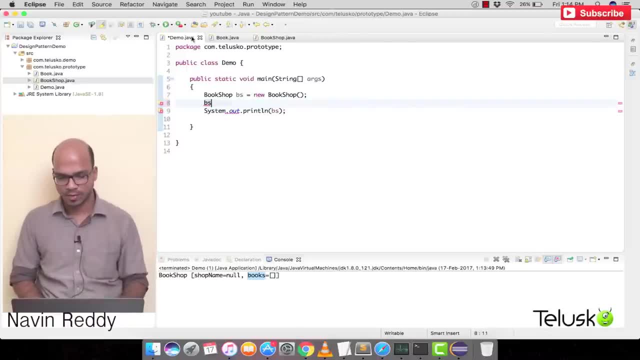 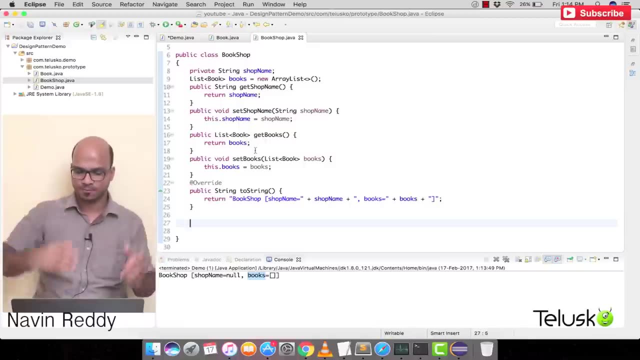 now there are multiple ways you can assign the values from here. or let's say, i want to fetch the data from the from the database, so all the book names will be assigned to the database and the book names will be coming from the database. so what you can do is you can create one more. 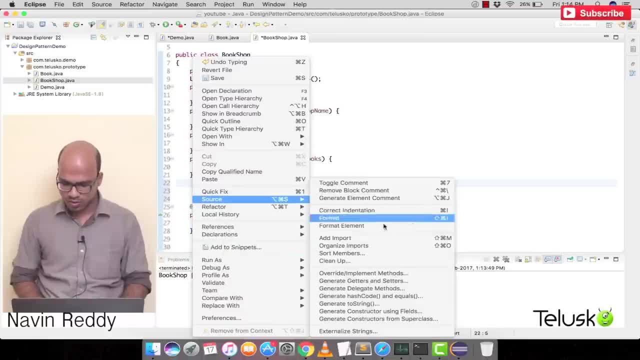 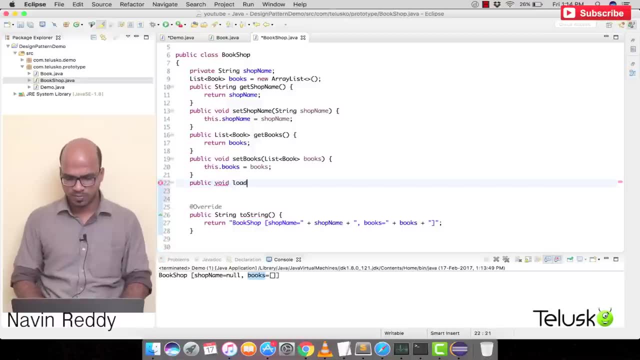 method here which is, let's say, write like source or not source. let's get a method by ourselves. let's say public, we'll say void and let's say this will say load data. that's your method name. now, what this method will do is it will add the data to your bookshop. 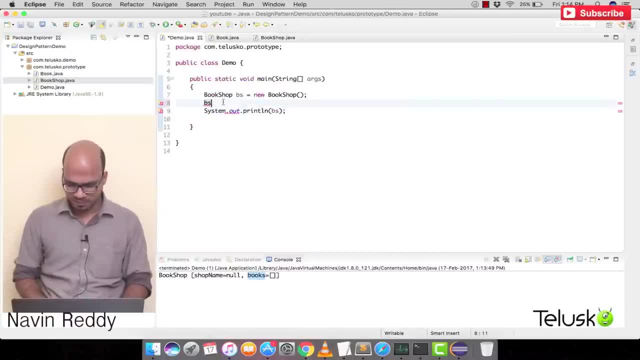 not the book name, because book name you can set it from here. you can say bs dot set book name. you can set that our shop name. you can set the shop name as novelty. i mean you can have any book, a book name, book shop name. i just have this shop near to my office, so i'm going for that name. 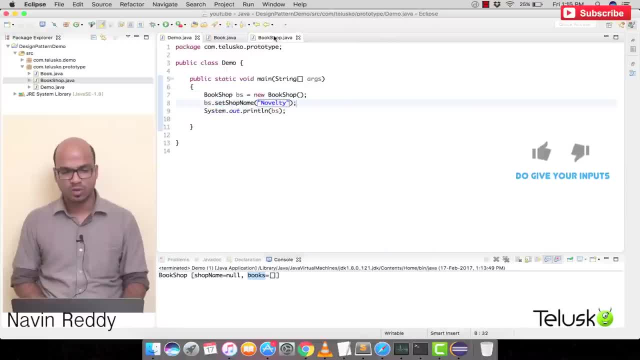 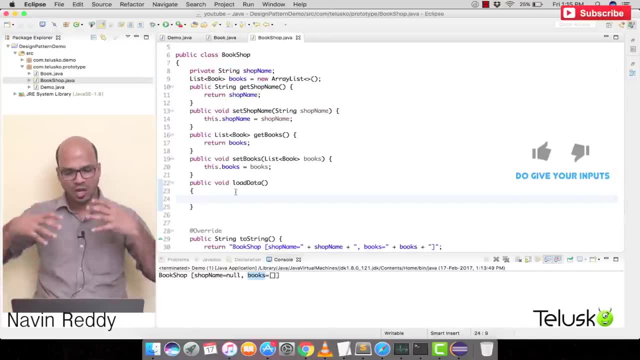 okay, so, but what about loading the data, loading the book names? so what you can do is in the in your book shop you have this load method and you. so now you will, you will do the database connection and you have to write those seven steps and you will fetch all the books from the database. 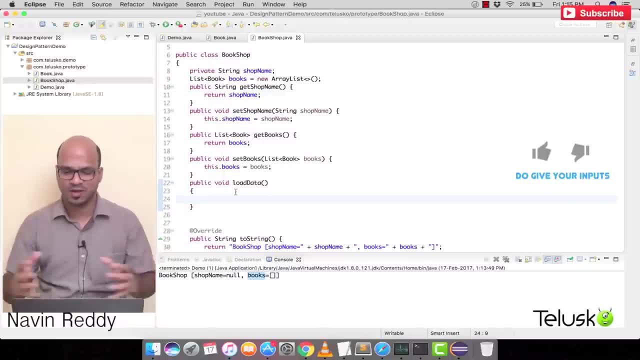 but let's say, if you don't want to use, if you don't want to go for database connection because it will take some time, right, because to write those code for demo purpose, we will, we will add those data by ourselves. okay, but just imagine if that is coming from database, how it will, how it look like. so let's use a for loop. 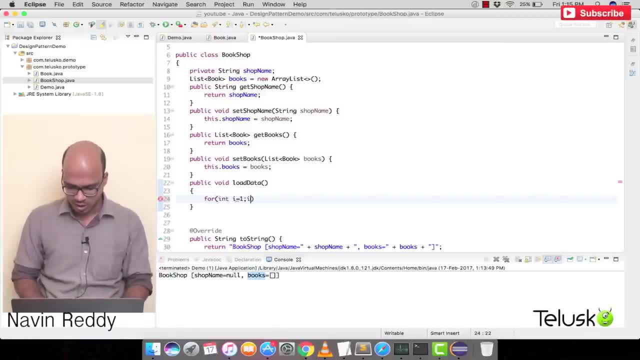 because i want to add lots of books. i want to add 10 books at least, so i will say 10, and then i plus, plus. i want to have 10 books. every time it this loop runs, i want to create object of book. we'll say book b equal to new book, and then, uh, we'll set the values for that. we'll say: 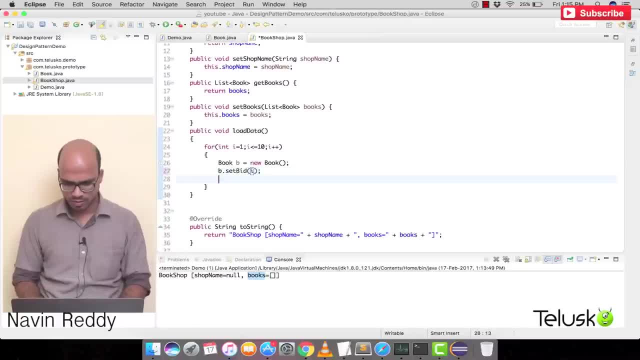 book dot set b id as i and b dot set b name as book plus. i right. so it will be having book one, book two, book three as names and once you've got the books you can simply add those books into your collection, so you can say, get books which will give you the collection of books. 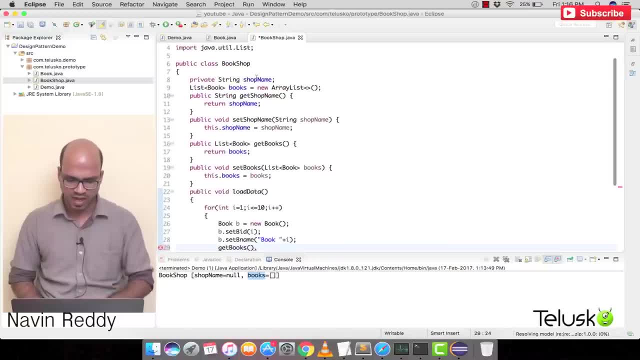 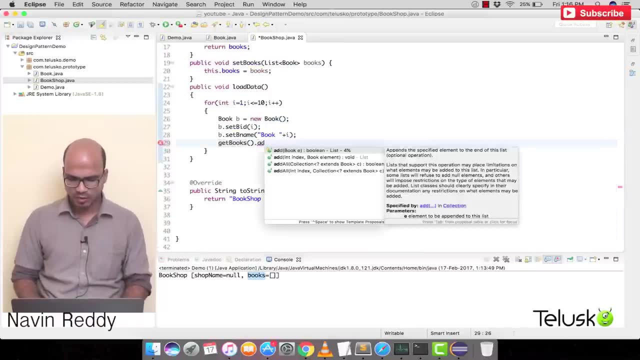 which is the list of books. uh, you can see we have list of books there, right? so we have list of books which we can fetch, that, both those books with the help of get books, and then we can say add and you can mention the book name, which is b, right, so it will add 10 books into your thing. 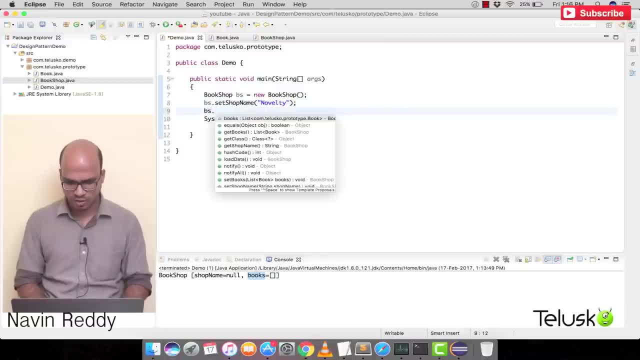 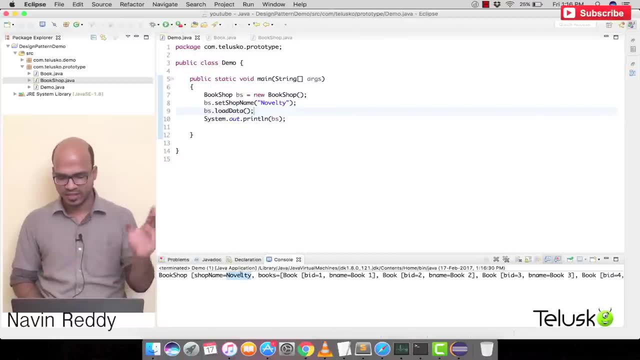 and from demo. what you can simply do is you can say b, s, dot, load data. so once you say load data, it will add all the books there. and now, if you run this, you can see we got the shop name as novelty and then we got all the book names here. you can see the list here, right? so we got all the book. 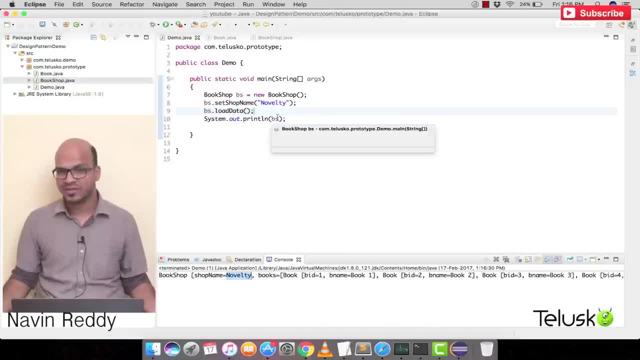 names. is that simple? but then where is the product design pattern here? nothing we have not done yet, right? so what i'm, what i want, is just to show you that the power of product design pattern. what i will do is i will get one more book shop. i will say book. 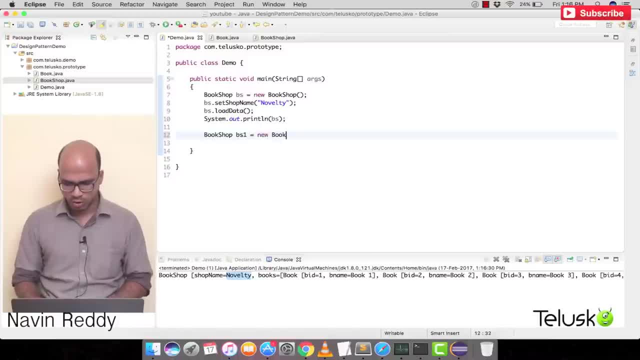 shop object. we'll say bs1 equal to new book shop. okay, it will. so this is your new object and, of course, if you print this book shop, you will get the same output, which is blank, right? if i run this code, the first line, you will get all the data. the second line, you can see it is null. 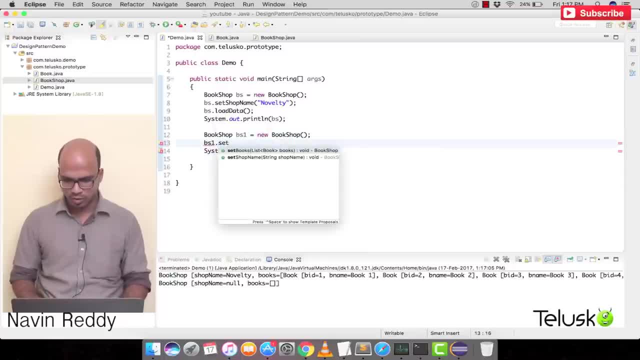 we have not specified the name, let's do that. we'll say bs1 dot set book shop name. i will say the shop. okay, that's your shop name. so you can see we got two shops here, two book shop, one with novelty, one with a1. but a1 doesn't have a book, right, so we have to load the book. so what again? we have to. 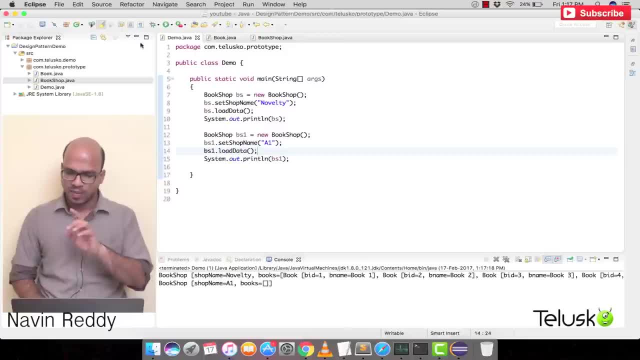 do is we have to say bs, i mean bs1 dot, load data. but the moment you do that, if you load data again, it will go to database. it will fetch the data. it will take some time, right? so instead of fetching the data from the database, what if we can simply ask: hey, bs, can you give me your data? is it possible? 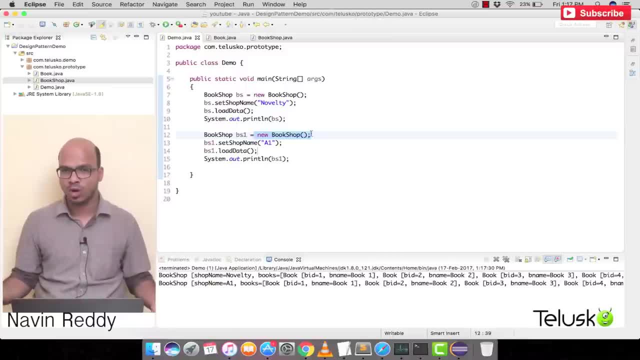 what you can do here is, instead of saying new book, you can simply say bs, dot, clone. so we have a concept of clone in java which can copy the data for you, which will create a new object from the old object. so you can simply use clone, but unfortunately we have two types. 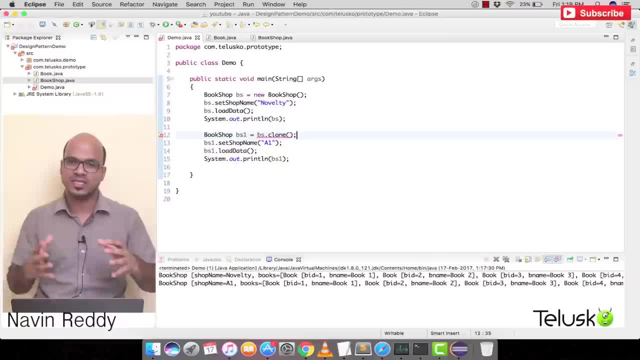 of cloning in java. one is shallow cloning and second is deep cloning. so when you say bsclone, it will go for shallow cloning again. but the problem is it is not working. here you can see, it says the method clone from type object is not visible. the problem is this: 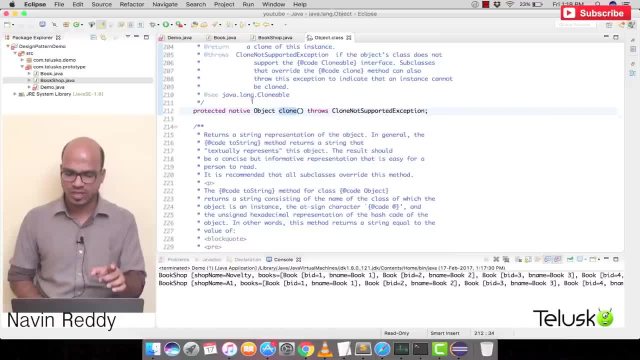 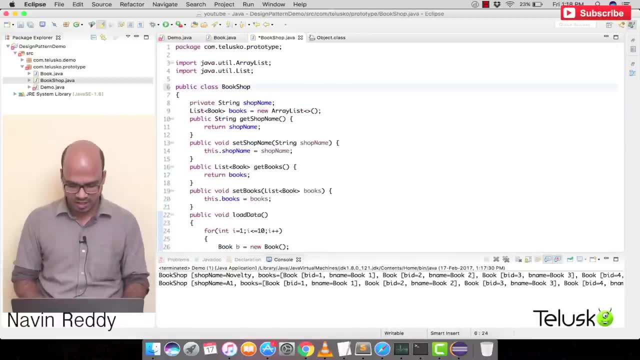 clone method is there in the object class, but unfortunately it is protected. okay, you cannot use that. so the only way you can use that is by, first of all, you have to give permission to your class. so your book shop needs a permission that you want to. you want it to be cloned, so you have. 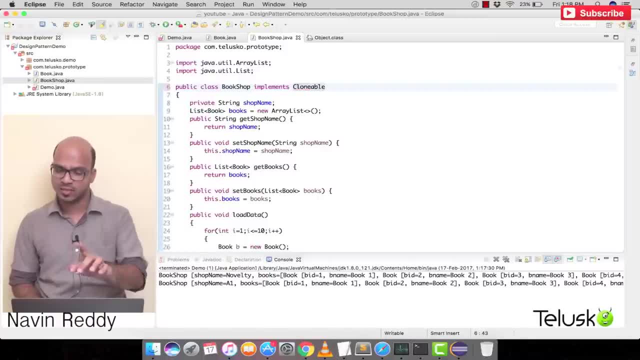 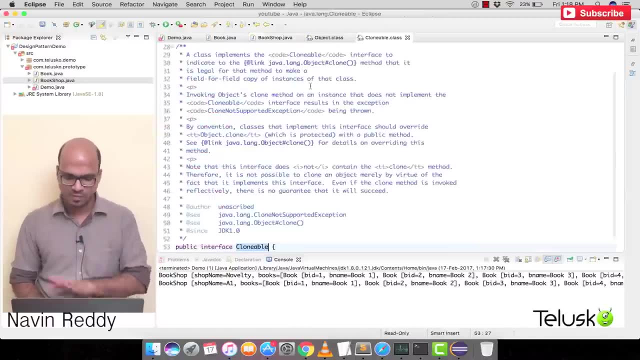 to implement an interface called as clonable, because if you don't do that, you are not allowed to use that. okay, so you have to make sure that you implement a clonable interface again, this clonable interface doesn't have any method. okay, this is a marker. 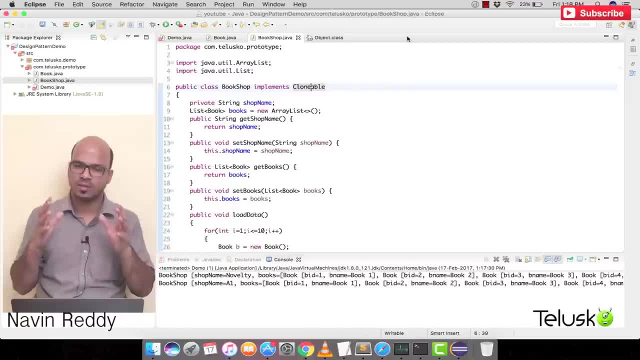 interface. but still so, what is mark interface? uh, basically, if you have, if you don't have any method in your interface that is called marker interface. okay, so this clonable interface is: we are just implementing that, so that will give the permission for the book shop that it can be, it can be cloned. 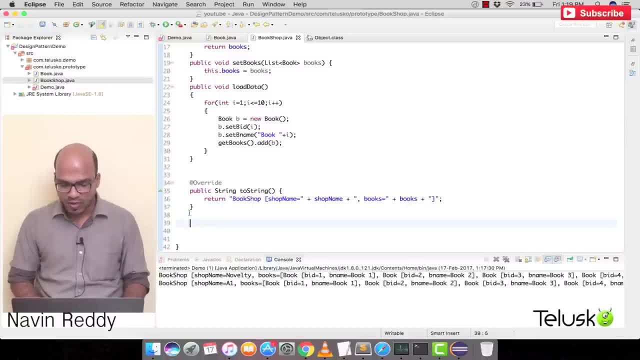 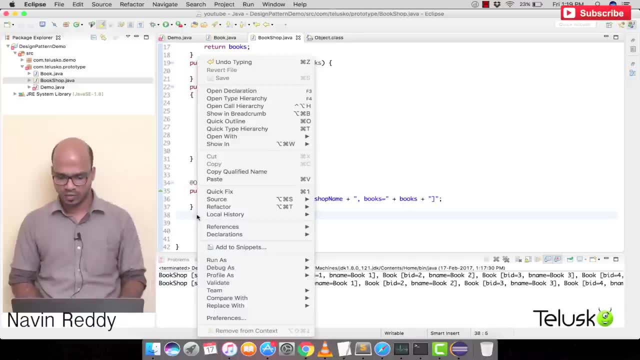 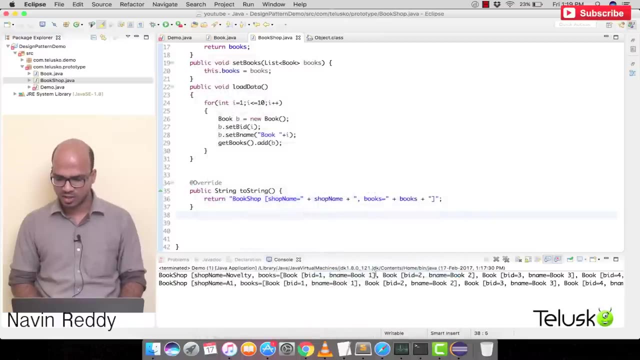 but then to achieve cloning, we have to override a clone method because, again you can see, it is not a clone method, okay, so if you want to have a clone method, you have to override it, and you can do that by using get source and you can see this option of override implement methods. click on that and 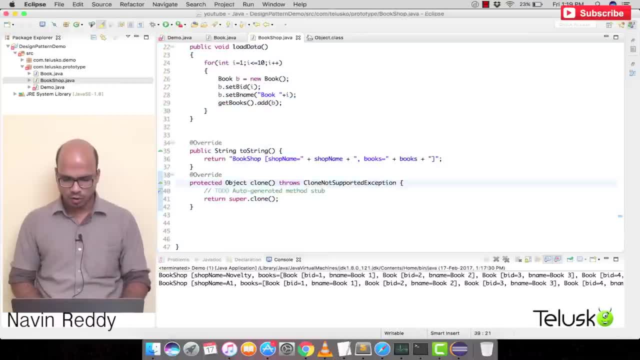 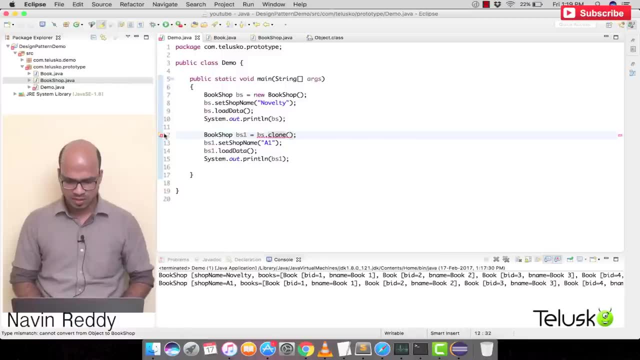 you want a clone method, just click on clone and click on ok and you can see we got our clone method and our job is done right. and if i go back here, okay, it is giving me an exception, let's okay, it is not giving the exception, it is giving you the problem. so the clone method will. 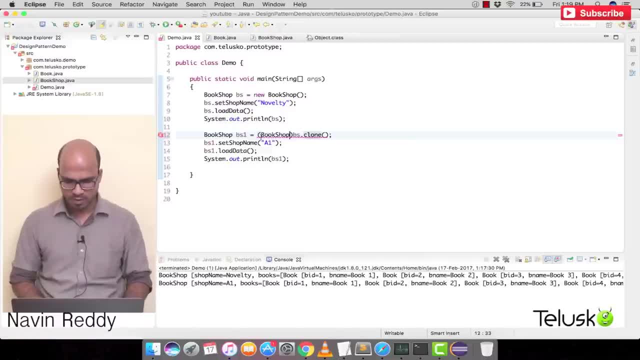 i want to convert that into a book shop type. right, that problem is solved and it also might throw an exception. so let's add a declaration which is a clone, not supported exception, because it will throw the exception. if you don't do this, you have it is compensating for you to 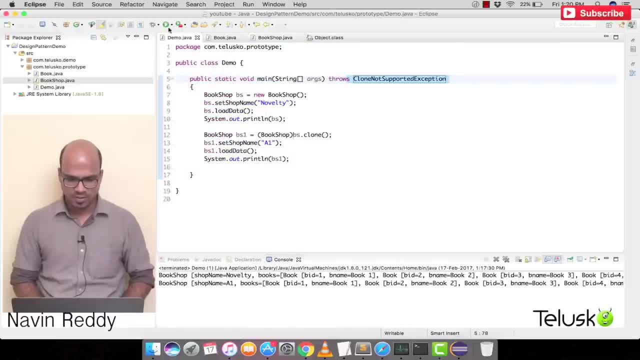 implement a clonable interface. okay, now let's run. let's see what happens if i run this code. oh, it worked. can you see that we are not creating? i mean, okay, let me just remove this thing. is it because of this? you're thinking about that? okay, let's remove. 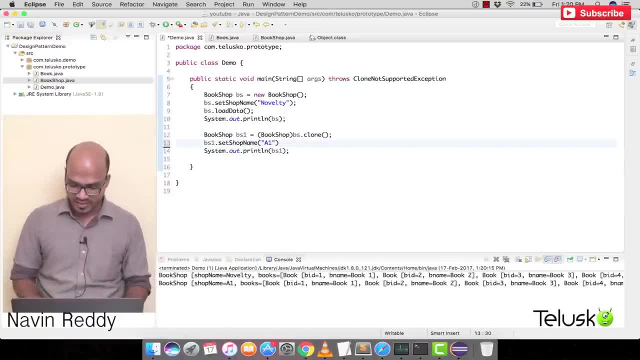 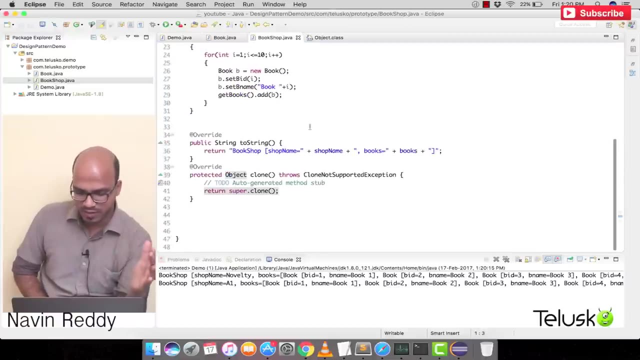 that, and so it works. you can see, even without loading the data, you are getting everything simple, right. but there's one problem here. okay, the positive thing is you got the data without using a new object. you can simply clone the object. the steps are: your bookshop need to implement a clone. 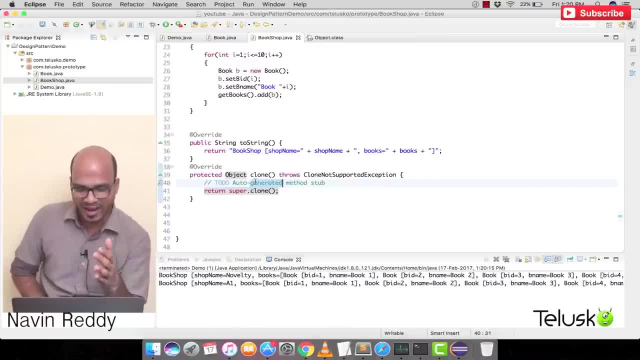 method. again, you don't have to type anything. you can ask your eclipse to do that for you. and second, you have to implement a clonable interface. now, if you look at this code, how do we get a clone method? okay, so let's say you have a selected object clone because it returns an object type. we have to say: 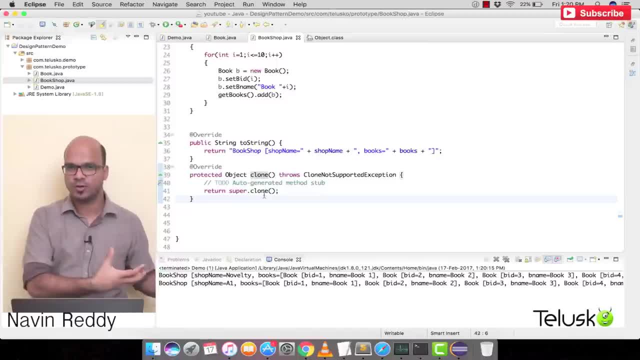 clone and then you simply have to say superclone. okay, so internally it will, it will create a clone for you. but the problem is this type of cloning, which is default, overriding the clone method, will give you shallow copy. now, when i say shallow copy, what it means if i go to demo and if i 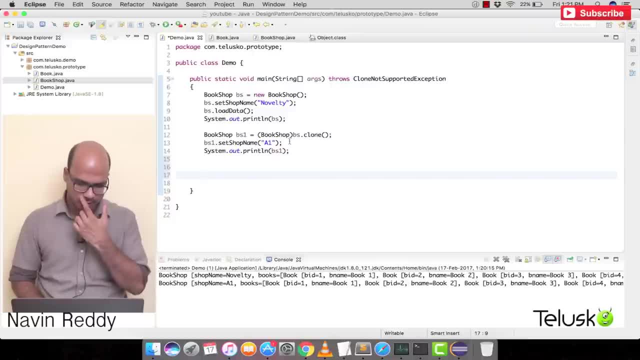 if i change some data, let's say, if i say okay, what i can say here? okay, let's say i want to remove one book with the index number two. okay, which is the second book or third book? right, if i run this code, it will remove the third book from the first one, from the from bs. 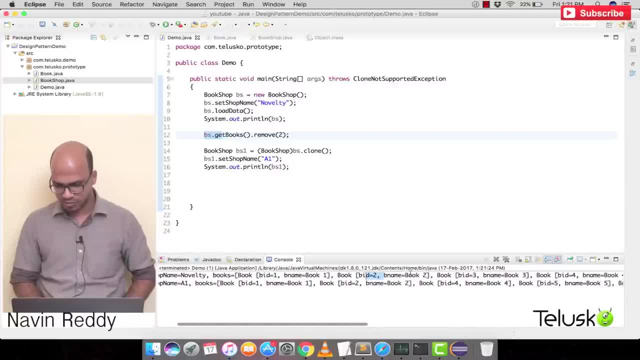 you can see: we got bid one, we got bid two. we got bid three, but okay, it is not. it has not removed, because i am removing that after the printing. okay, let me just do that before printing my mistake. okay, you can see. we got one, we got one. we got two. we got one. we got one. we got two, we got. 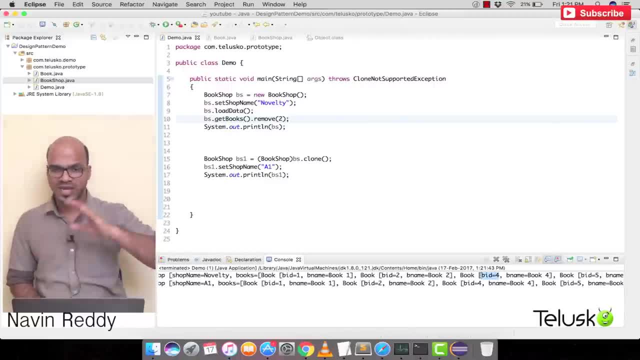 two, but there is no three here. we directly went to four because that means we are removing that data from there. but it is also affecting bs1. can you see that in bs1 also we don't have, we don't have three. now it is directly going for four. that means it is not creating a new object. 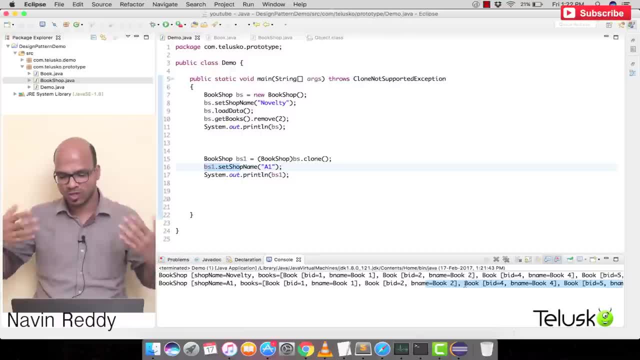 for you. we just have one object and we have two references, so cloning is not that impactful here. but then question arise: how to achieve deep cloning. so in deep cloning we actually create two objects. we have two different objects and they will have two different data. okay, so one. 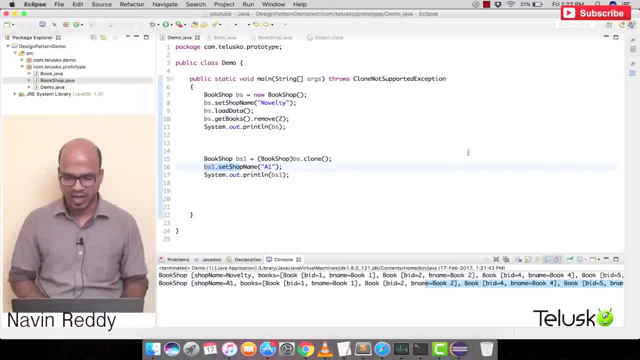 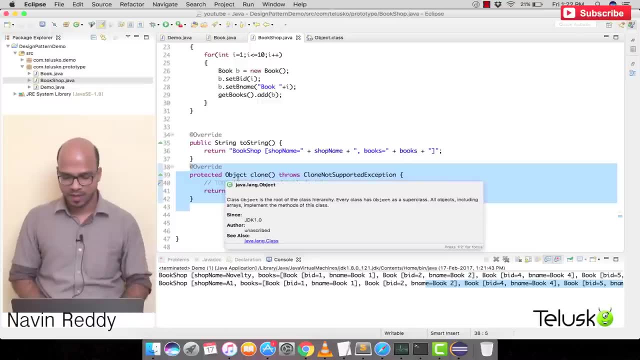 object will not affect other, so it's always better to go for deep cloning. but how do we do that? it's very simple: just go to your bookshop and say, hey, i don't want to go for normal cloning, i want to go for deep cloning. in that case, since you are changing the definition, we can. we can change the. 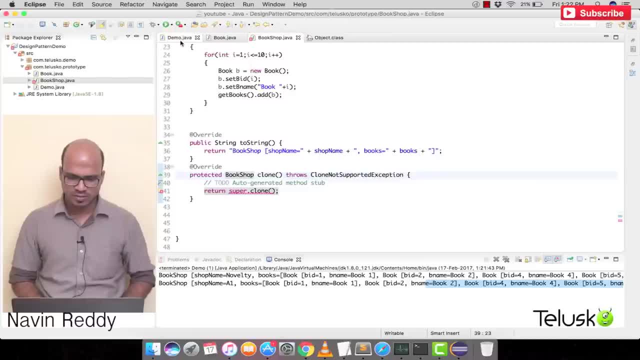 return type. we can simply say: i want to return a bookshop. so once you do that, let's go to demo and let's remove this casting. we don't need a casting now because you are returning a bookshop object, but then in here you cannot do this, you cannot return. 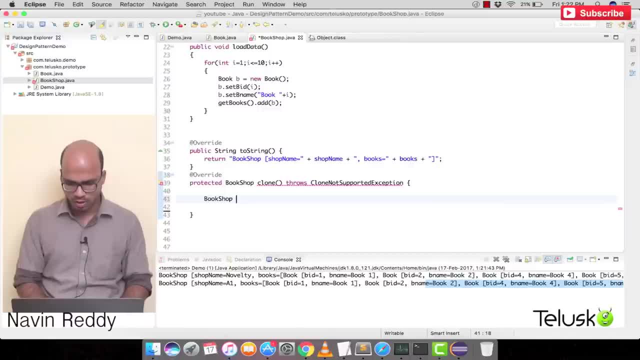 so what you have to do is you have to say you have to create a new object. here. we'll say bookshop bs, equal to new book shop, right, we got an object there. and then we can simply set the. let's not set the book shop name here. that will that we can do later, but we can return the bs object name. 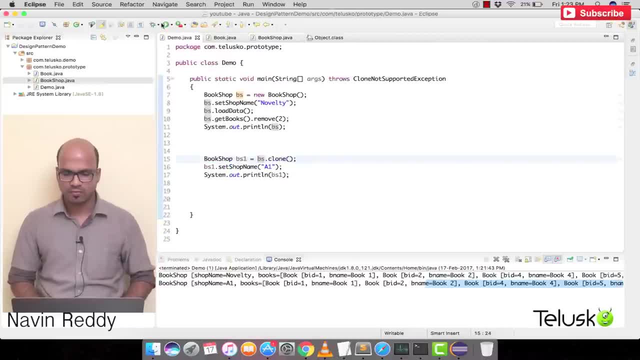 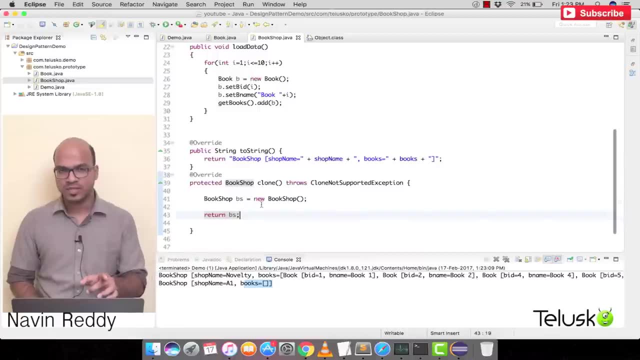 but then this will not work right, because if you run this code- i mean of course it will work- you will get the output, but the data will be empty here, because we are returning a new object which doesn't have a value. so let's assign the value there, since we already have a value. see, 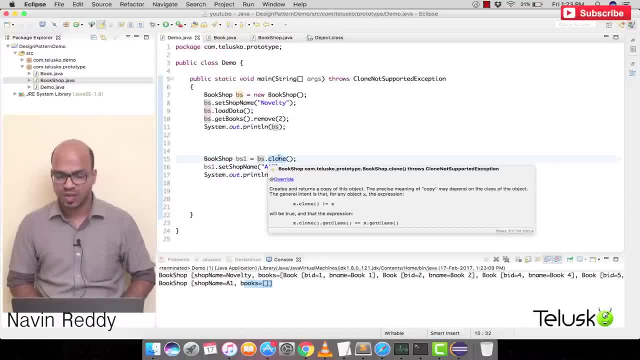 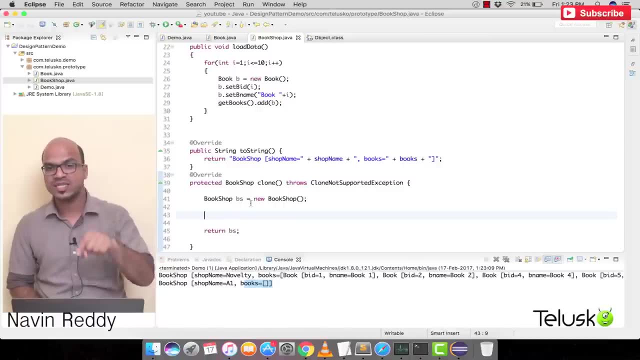 when i'm calling this object, i mean when i call this method clone- i'm calling that method from bs object, right? that means i can access that bs object here using this keyword, right, because that is what calling the clone method. so what i can do is i can use a for loop and we can fetch the value. 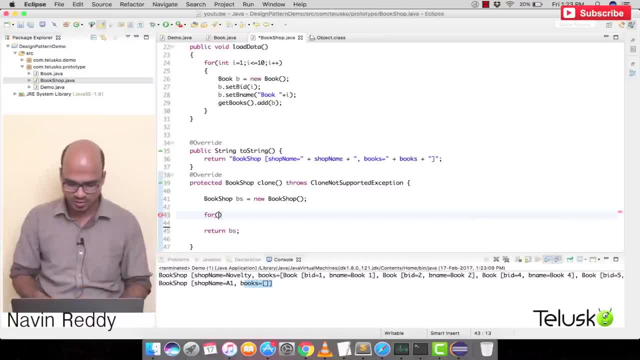 from bs object and we can put that object into new object. so how do we? how do we do that? we'll say: uh, book b, colon, get books. Now, when I say get books, I am actually talking about the object which is bs in here. Let me change this name. we'll say: this is shop. just to make it simple, let's. 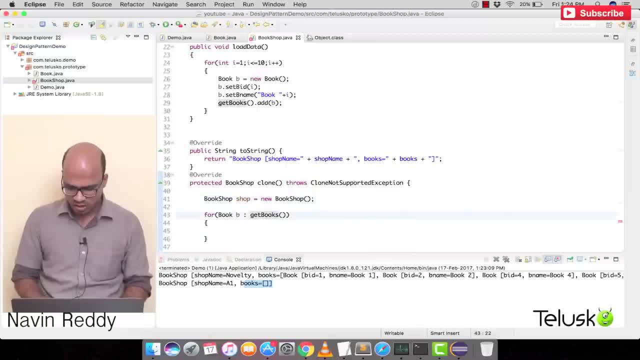 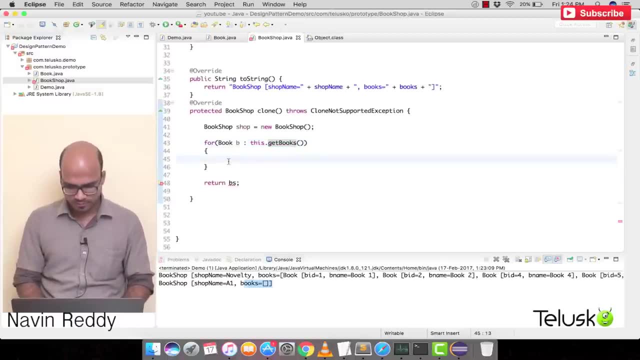 make it shop. Okay, so we can also use this dot get books. that will make that will be better, right, Then what we can do is we can use shop dot get books, dot add, and you can add b here. So what we are doing is we are using a for loop and we are fetching the data. 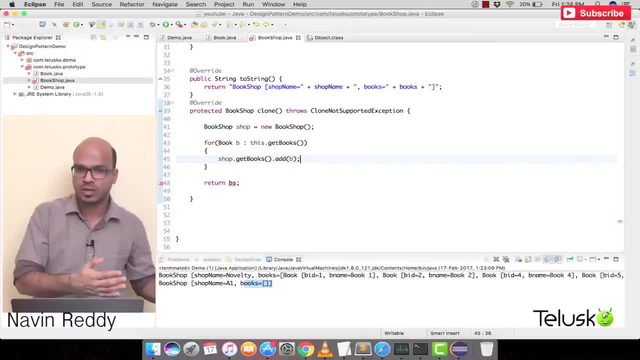 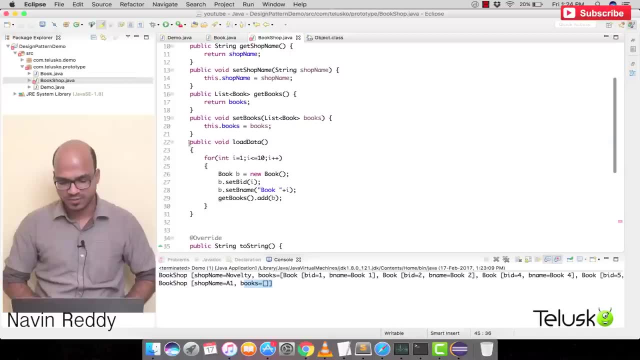 from the old object and fetching one, one name and we are assigned a new object. Then you will say we are doing the same thing, right? not exactly. This load data is fetching the data from the database. So for bs object, I mean for the first object you are fetching- 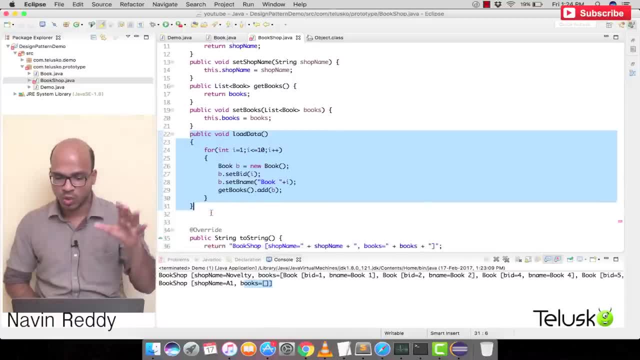 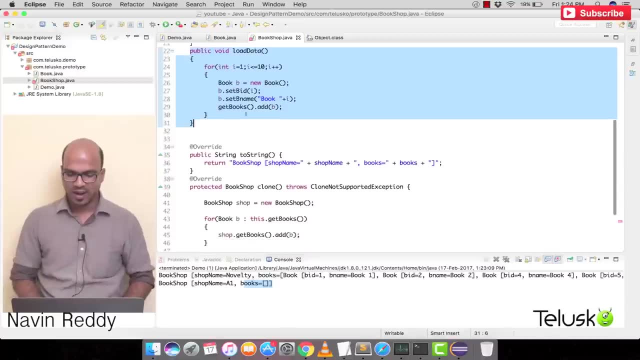 data from the database. for the second object, you are not fetching data from the database. you are fetching data from the old object, which is much faster than comparing with the database connections. right, And it should work. now let's run this code. Okay, we are getting an error there, I guess. 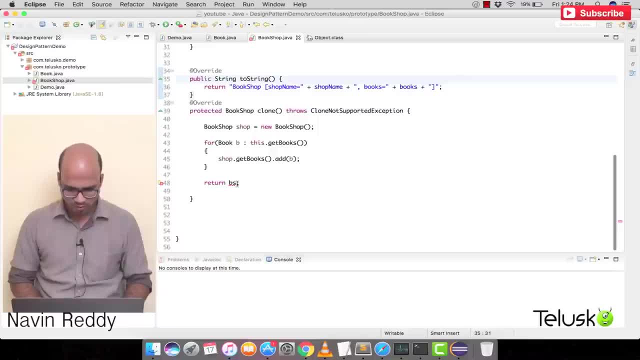 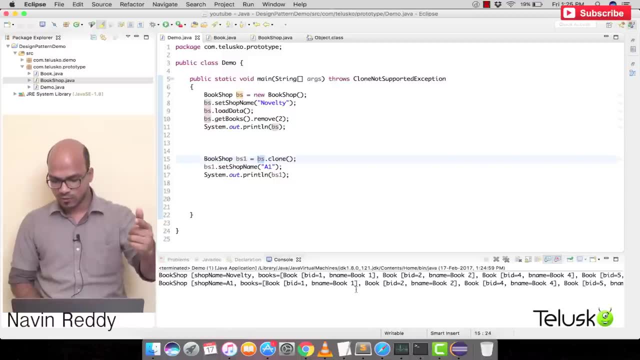 we have an error and the error is with this line. we have changed the book shop name, right, so it is shop, And now let's run this. can you see that we got the output and again we got a problem. So the problem is okay, we are cloning that after removing that. okay, 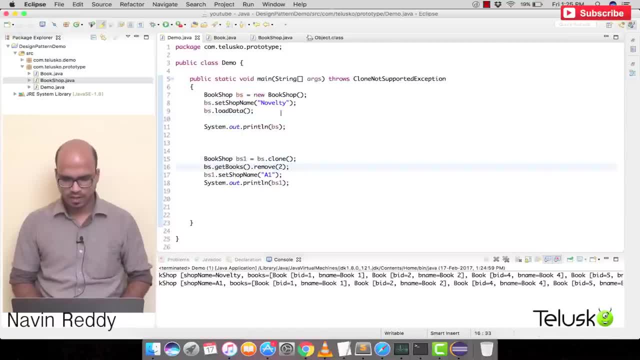 what I will do is I will clone it after this. Okay, so I am cloning it and then I am removing the data from bs. You can see it is not affecting your third one. instead, I should print this. I should print it together. both the objects will be printed together, so that you know. 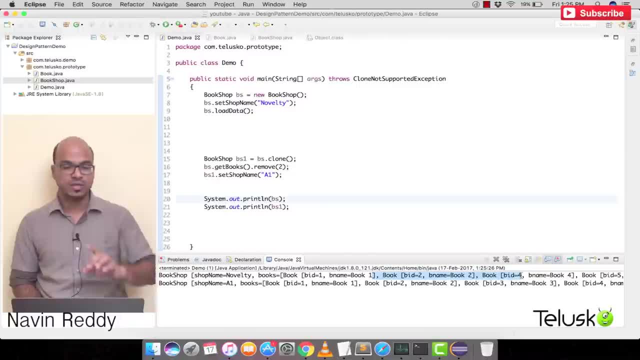 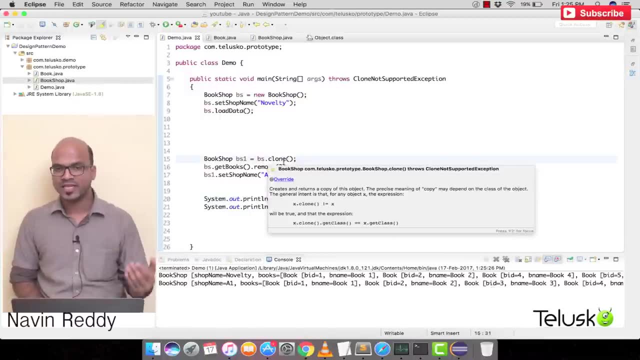 it will not impact. So you can see, in the first object it is affecting it is removed 3. but in the second case it has all the data: 1,, 2,, 3,, 4, okay, So that's the advantage.